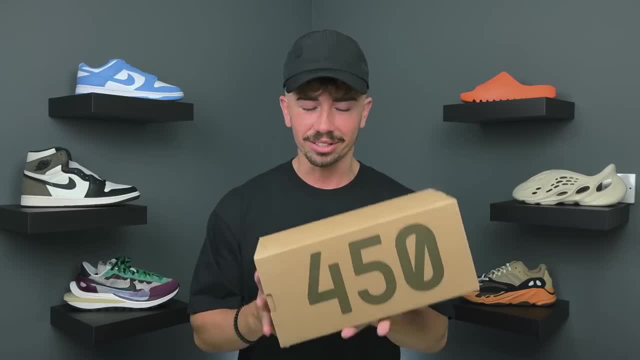 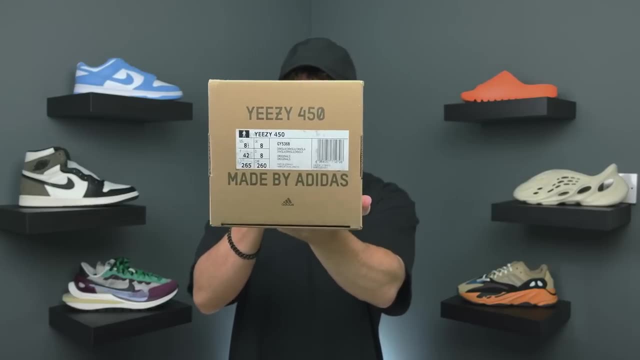 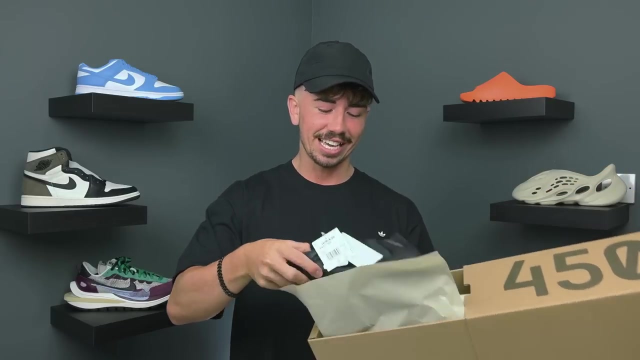 We got the Yeezy 450 box, The small compact kind of cut in half box. So take a look at the size tag before we slide these open. and take a look at the dark side of the Yeezy 450 and that is this one right here, The dark slate colorway. Of course, the 450 always comes out of the box looking all squished. so, yeah, it's not the best first impressions, But generally speaking, I think the Yeezy 450 has been accepted pretty well by the sneaker community. I mean, it's kind of a symbol of bold creativity. Kanye starts working for Nike. 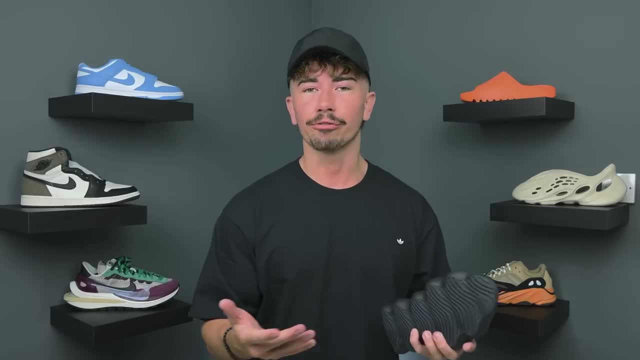 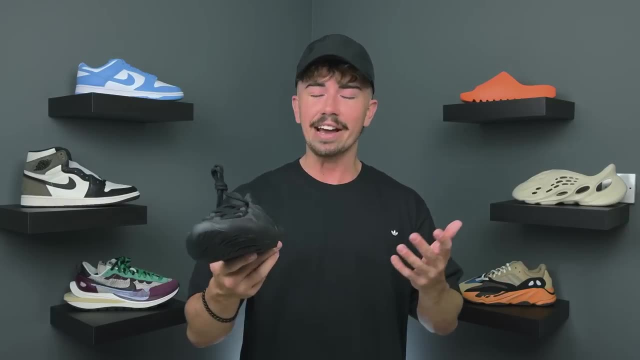 a huge company and they don't allow him the creative freedom to be able to create a lot of the ideas that he has. Adidas opens their doors and allows Kanye to create things that he never would have had the freedom to do over at Nike, and he has created a billion dollar company. 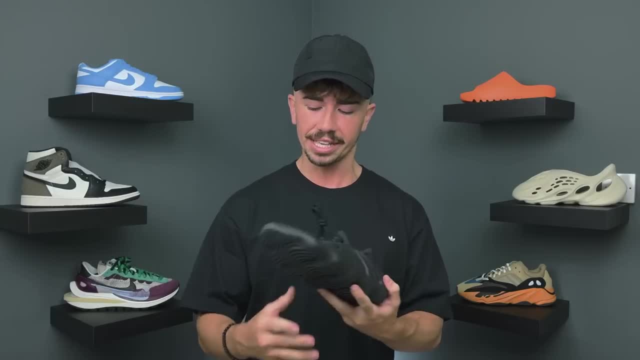 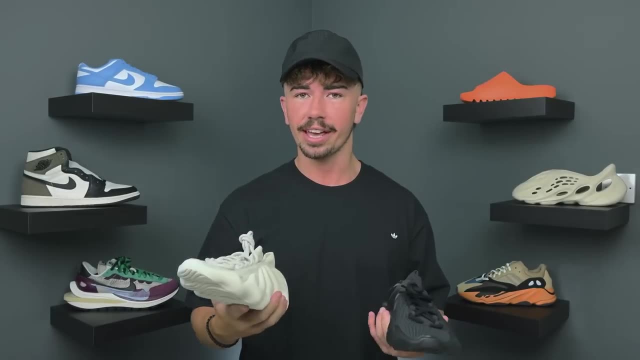 So, like a lot of introductions to Yeezy models, we get an initial colorway which tends to be on the lighter side, for example the Yeezy 700 v3 which came in the AZIEL colorway, And then the second colorway, which was the darker ALVA colorway. 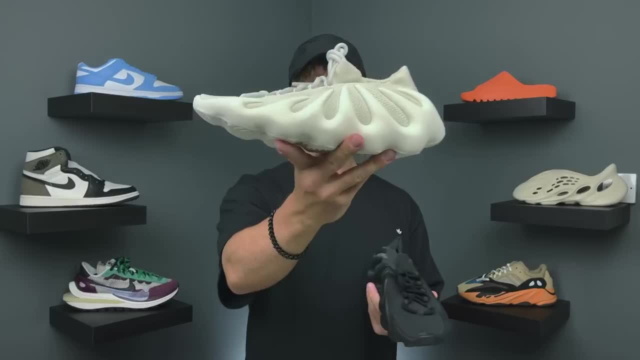 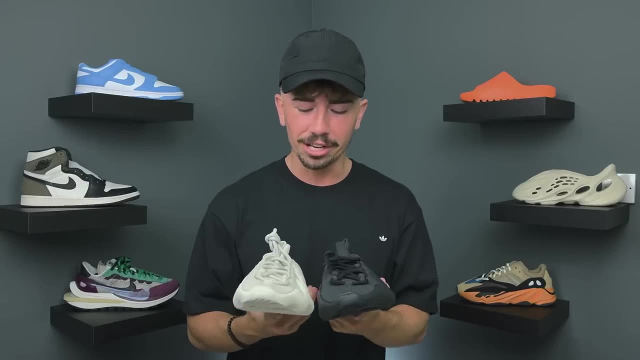 We're getting that same treatment over here with the Yeezy 450.. This cloud white, which initially released earlier this year, and now we have the dark slate. So really I don't even know if it's necessarily a question of which one is better. 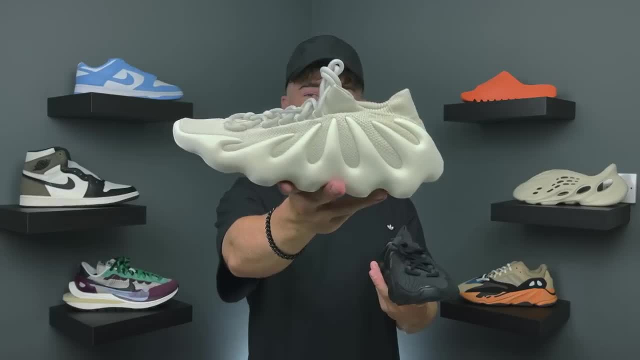 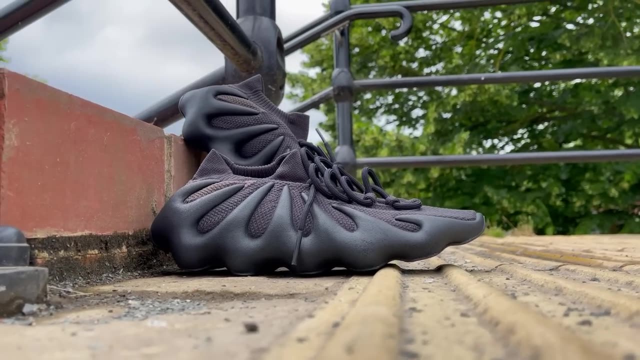 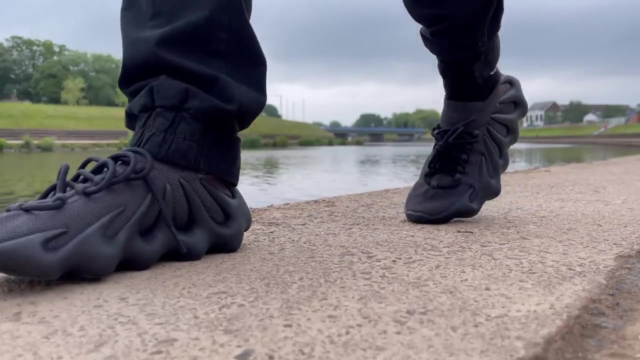 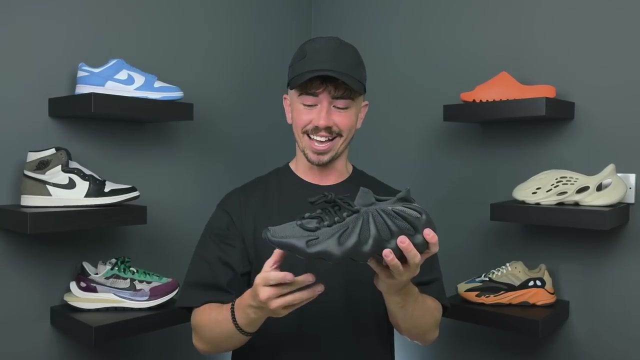 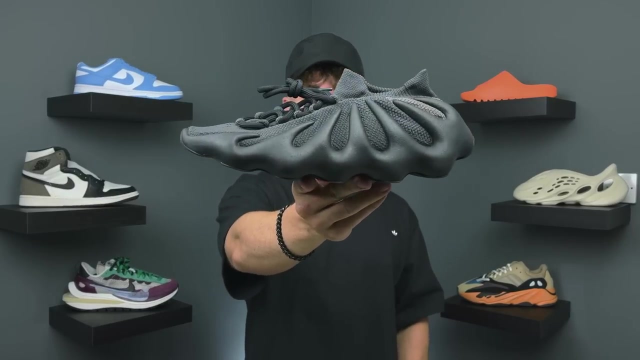 It's just, which one do you prefer? do you prefer? Do you prefer lighter colors, or do you prefer darker colors? I do have to be honest, though: this dark slate colorway is a lot nicer than I originally anticipated. Once you get this in hand, it looks pretty damn cool. But before we get into all of 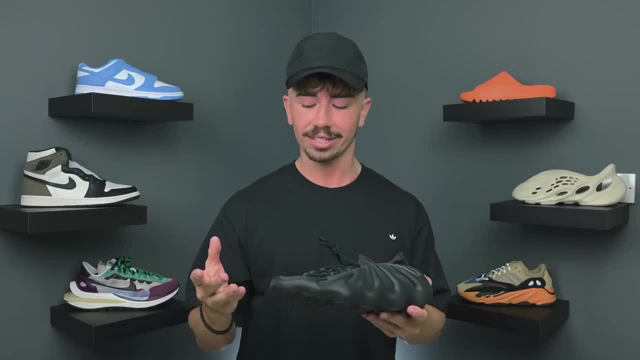 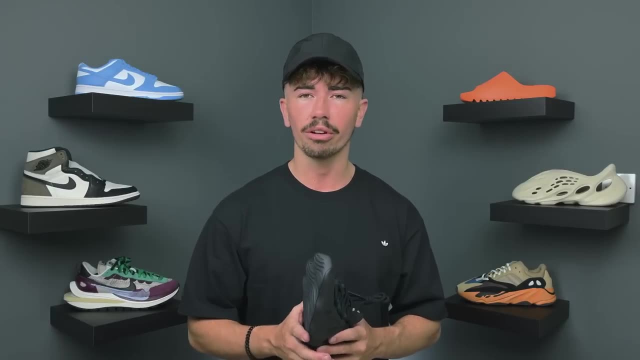 that, of course. let me give you guys some specifics on the Yeezy 450 dark slate. These released on Saturday, which was June the 26th. They retail for £170 here in the UK or $200 if you're out in the US And, just like the Cloud White release, both of these are already set to. 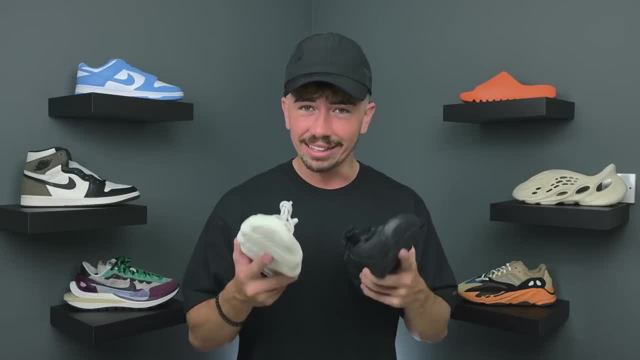 release again later on this year, But for there to be a rumored date the very same year of the actual release is something that is pretty different. All I know is that the Yeezy 450 dark slate is going to be released on the 26th. 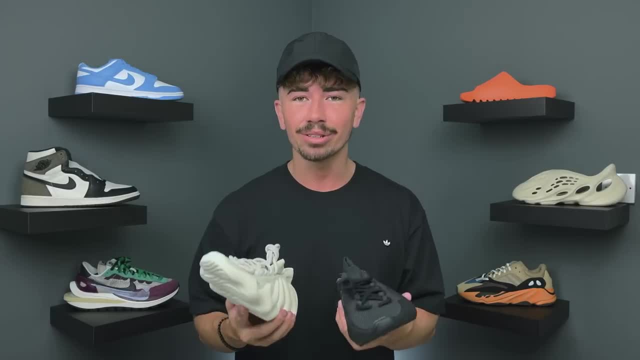 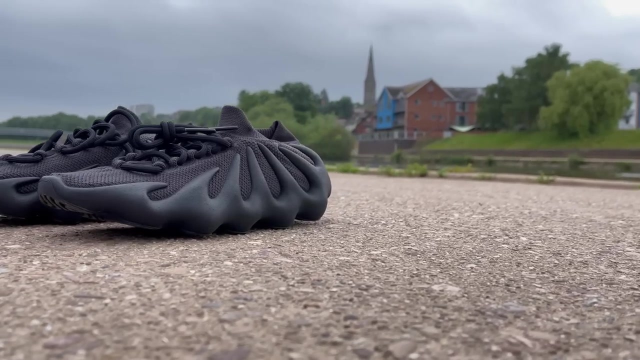 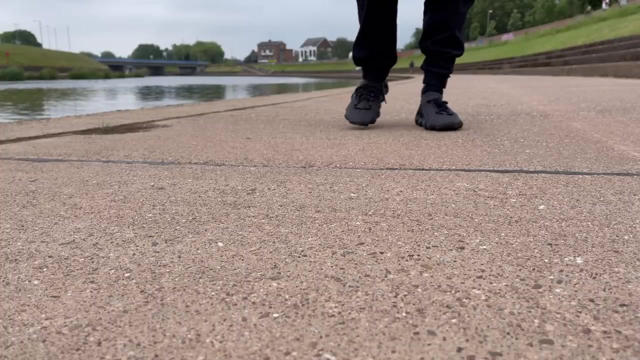 If you did take an L on either of these- September time this year or potentially October time- both of these colorways should be re-releasing And, yeah, you should have another shot at grabbing either one of these colorways. So, like I said, I'm liking this colorway. 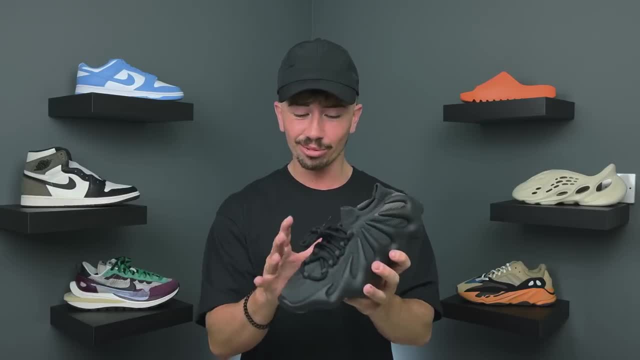 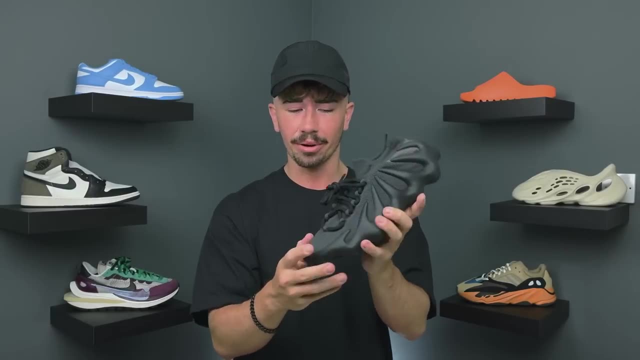 They did something really really cool with the colorway of this shoe. The upper kind of contrast really nicely with the midsole. So if you take a look at this knit upper you can see it's a little bit more charcoal. It's not completely solid black, It has a little bit of a lighter. 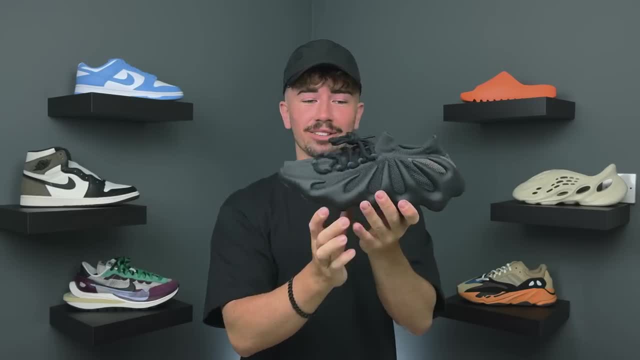 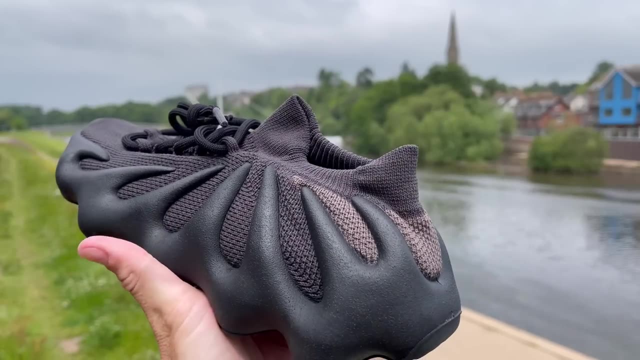 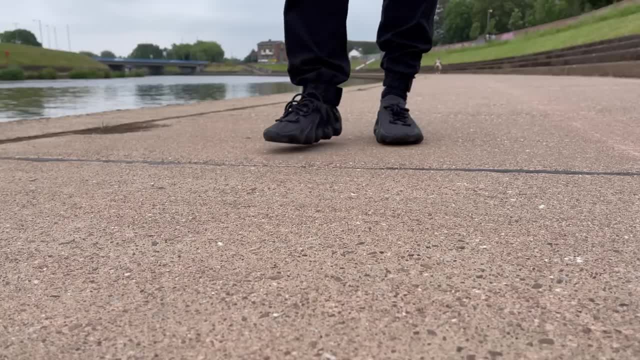 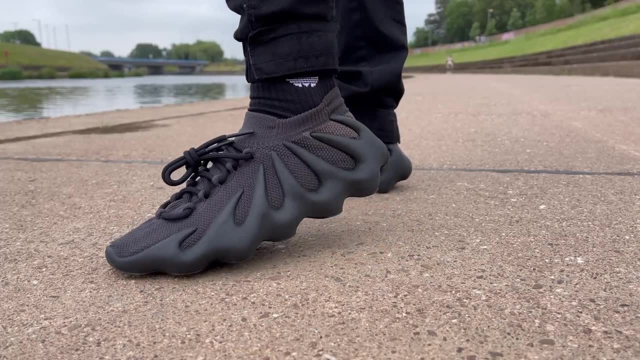 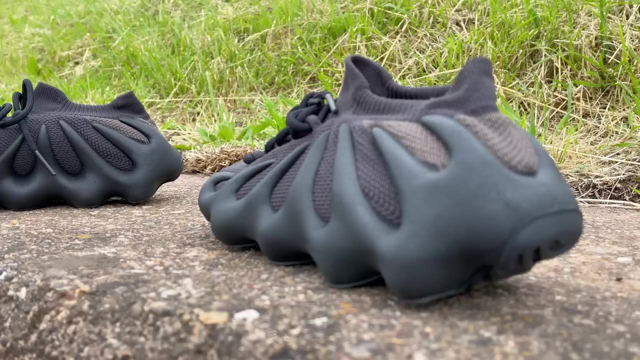 visible when you're actually wearing them. The laces that you get on here are solid black And the only kind of color change to this is around the back of the shoe, where you kind of find this little section here with a little bit of a brown hue. That's the only brown hue that you find. It might even be a little bit green. 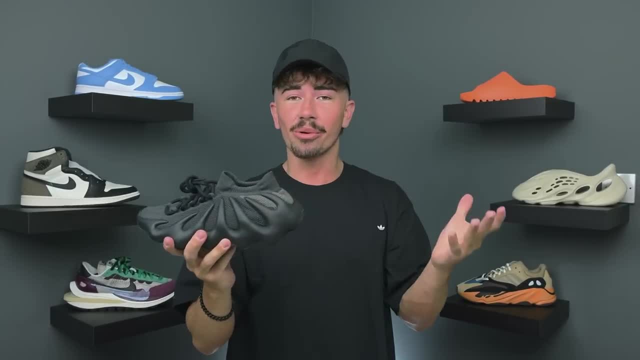 like maybe a very dark mossy green, but essentially that's the only other alternate color that you're getting on this pair of shoes, So that's the only kind of color change to. this is around the back of the shoes. Other than that it's a dark charcoal and solid black. 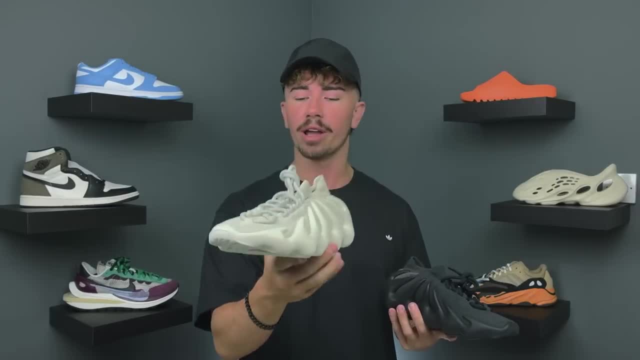 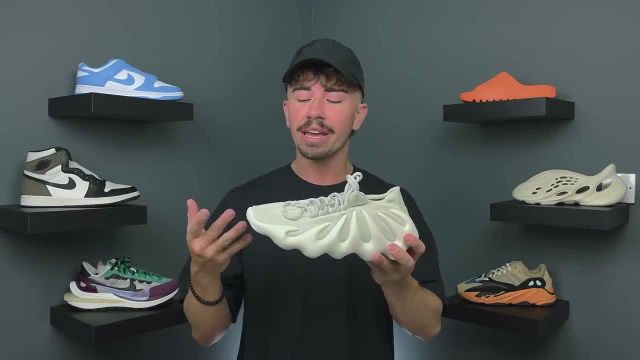 Now, obviously a big drawback with this original cloud white colorway was the fact that it got pretty dirty pretty quick. Now, obviously that's going to be conditional on how you're wearing it, But for the main part, of course, it being a very light, almost white color option, Yeah, 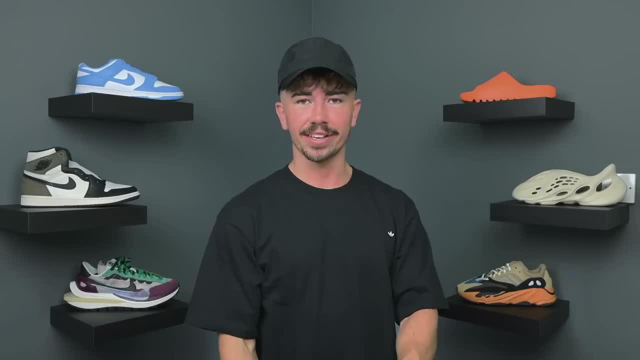 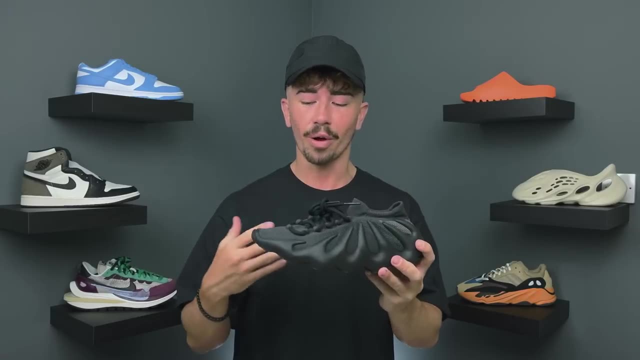 a lot of dirt is going to show up Now. the good thing about having a dark slate, a predominantly black colorway: it's going to be a lot more forgiving in terms of showing up dirt on this pair of shoes, So you can wear it and it will still look relatively brand new and you.